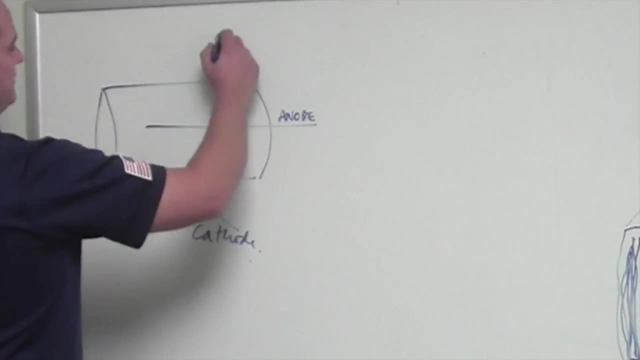 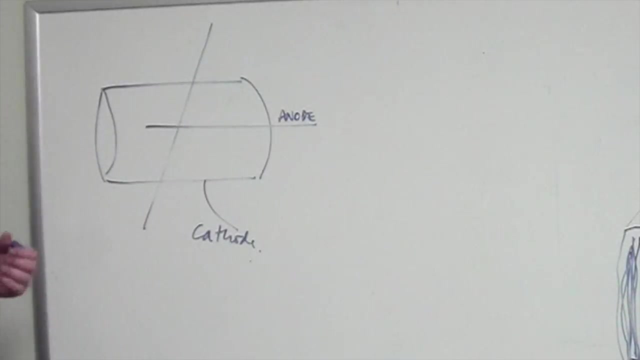 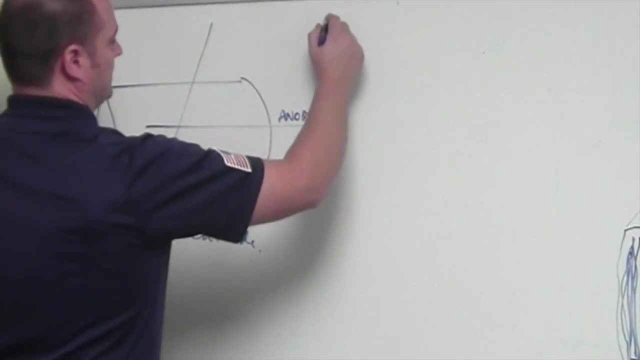 The whole process of detector radiation happens when an ionizing radiation, you know, particle on an x-ray or a gamma ray- crosses the volume of this cylinder. The cylinder has gas inside and it is polarized with a high voltage right, So you can have here, you know, 400 volts. 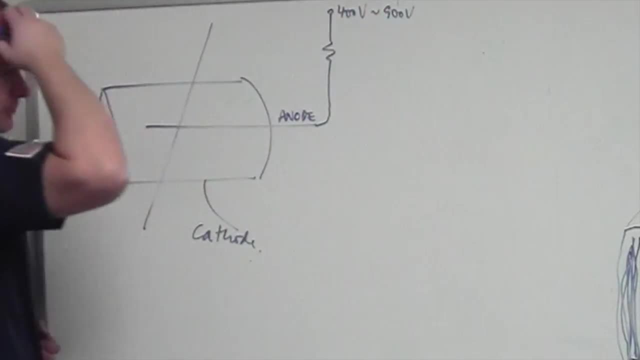 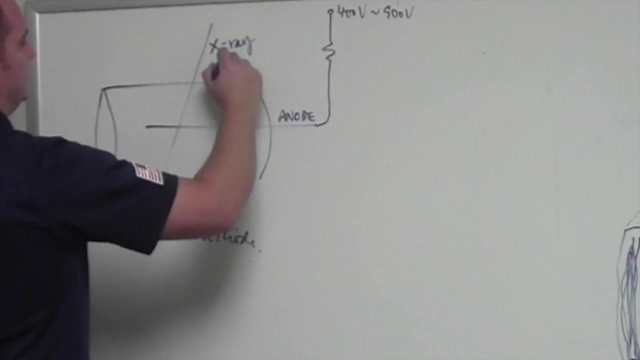 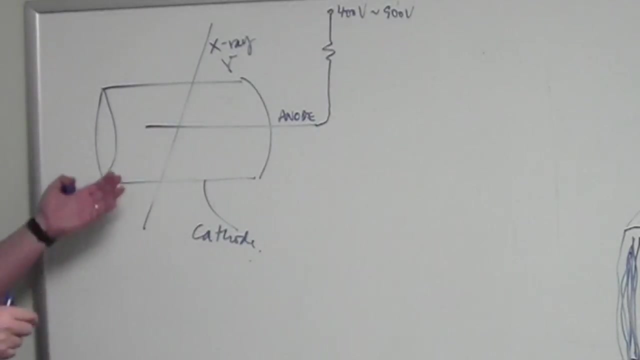 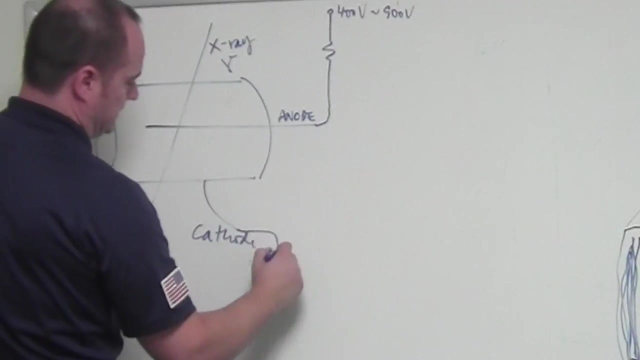 to 900 volts, depending on the GM tube that you're using. And so when this x-ray or gamma ray hits this detector, an avalanche of ions is created, which then creates a signal out of the cathode. So you detect the signal by putting a resistor here to ground, for example. just 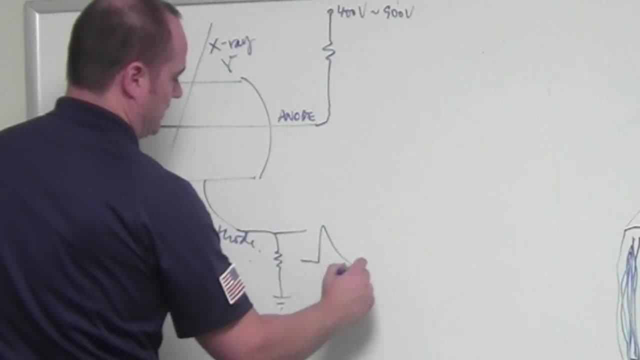 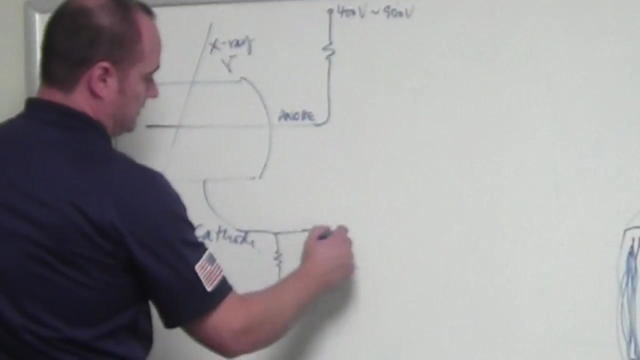 to a reference point and you're going to collect a signal that's going to be a little spark. if you will inside this cylinder, Then you know to get this signal, which is, you know, high voltage and it's quite noise, into electronics that you can actually 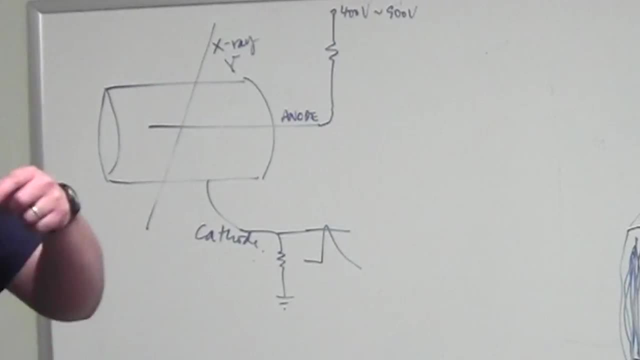 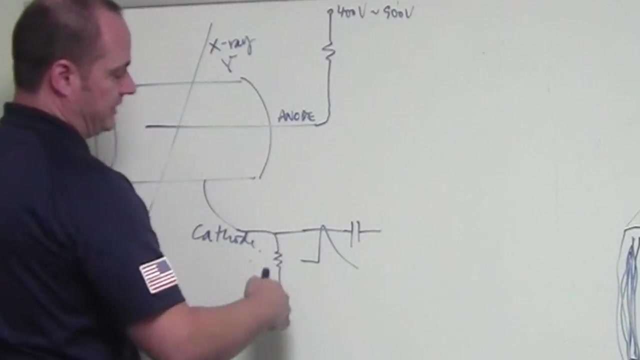 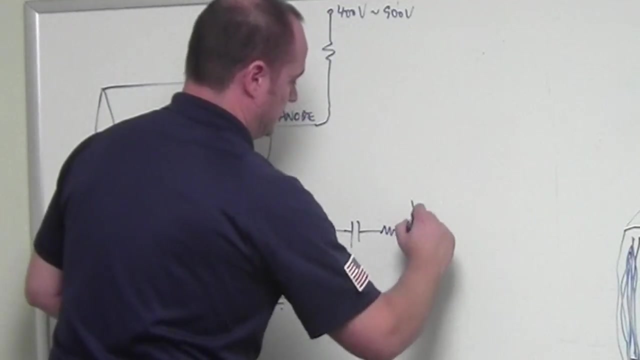 read into, you know, a nice display like this one. what you do, you know, the simplest form is just put a decoupling cap so that you, you know, get rid of a lot of the DC that might be coming from this circuit limit, and then just put a transistor here, that's. 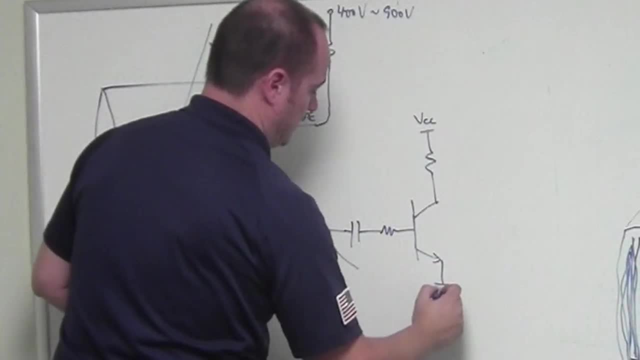 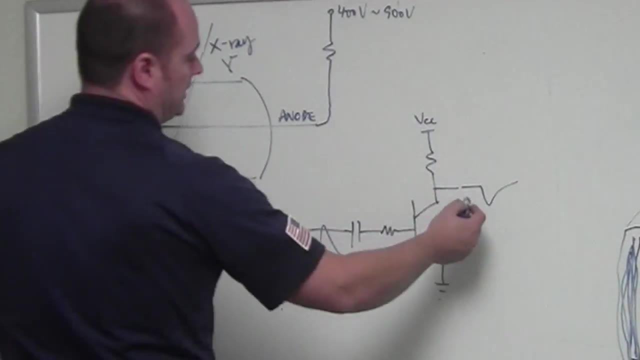 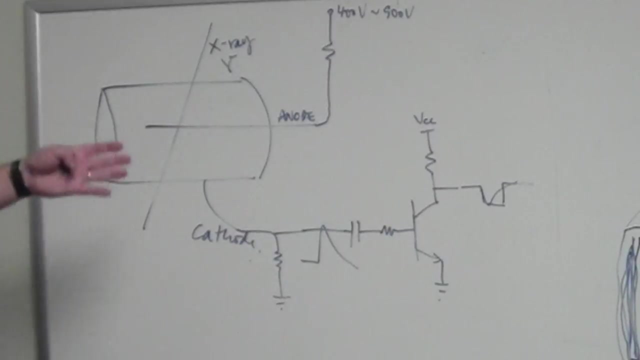 then put this guy to VCC, this guy to ground, and this signal is going to be inverted, of course. But from that point on you're going to have a wave that you can then take and read into your microprocessor. you can read into an Arduino, a PIC, whatever else circuit you. 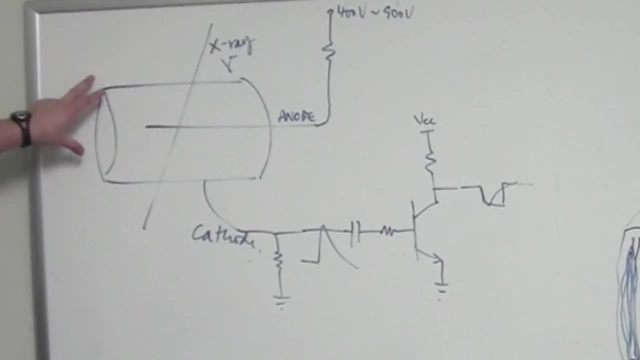 want to use. What's interesting is that the difference between this guy here: right, it counts particles, right, It basically gives you a hit for each X-ray photon that the cross is this volume. You don't really have information on the energy of that particle- A lower energy. 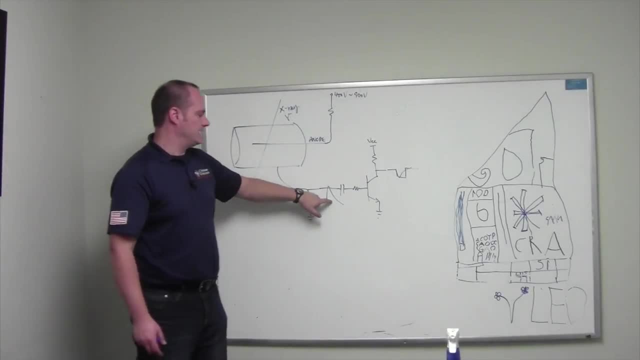 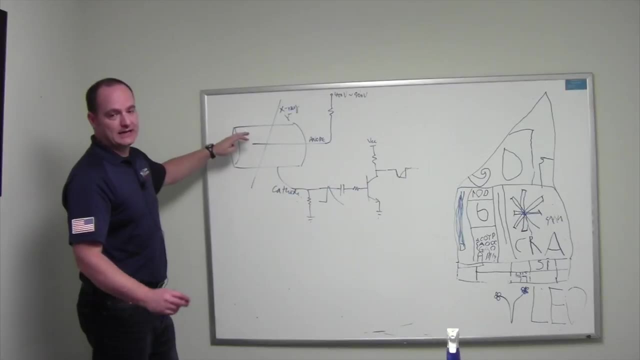 X-ray has the same. it's going to have the same signature as a higher energy X-ray. So this is not. it doesn't give you any spectral information on the radiation coming. that you're reading right. So there are other types of detectors, like scintillator detectors. 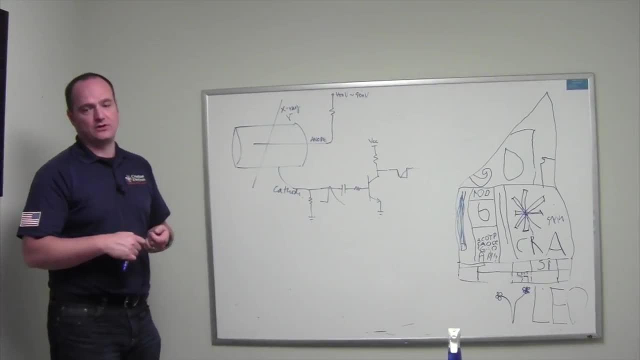 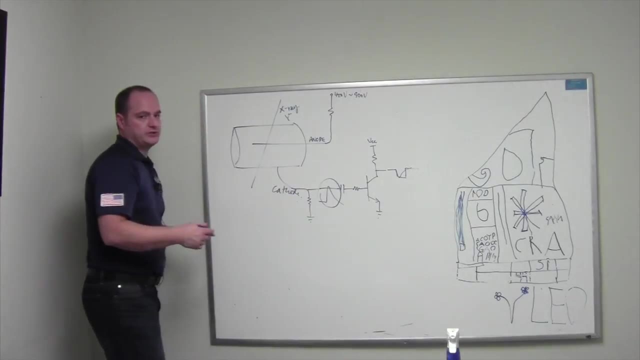 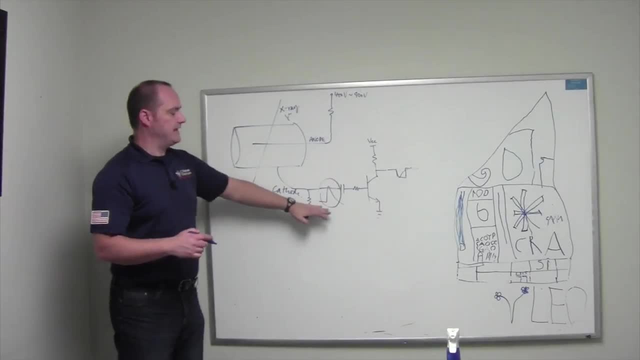 ray or X-ray hitting the detector And those then allow you to create a spectrum out of that detector. But again, this type, the GM Geiger-Muller Tube, will not allow you to do that. What you do is a reading. 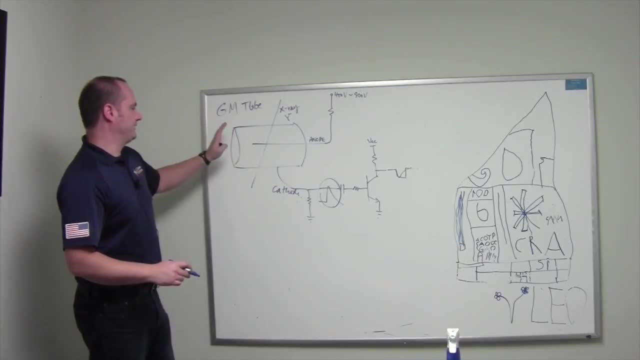 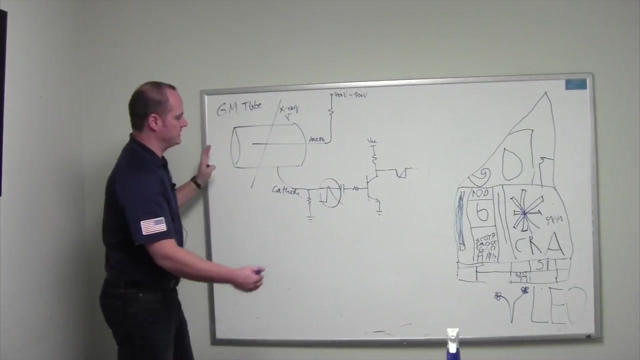 there is a variation of the response as a function of the energy of the x-rays or the gamma rays that you're reading, and now that's given by different manufacturers. There are compensated GM tubes, uncompensated GM tubes, but anyway, this is the simplest form, So we're gonna take this. you know this diagram and see. 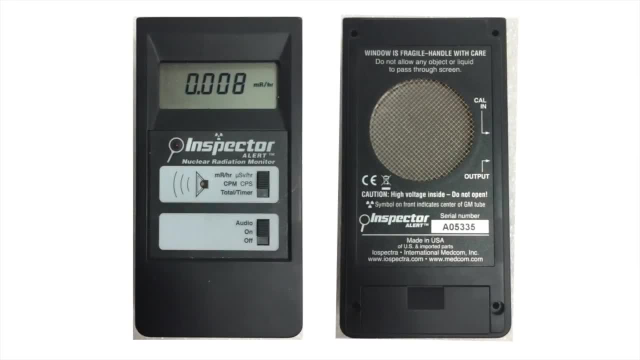 how we can map it inside this device. Okay, so now that we know how the GM tube and the Geiger counter works, let's take a look at the inside of the inspector alert. This is the outside box, as you can see, we have a display, we have some. 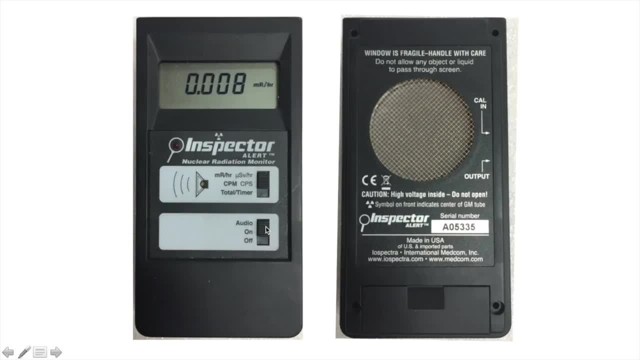 switches here, some selection switches- on-off switch, and another selection for audio- and then on the back of the unit you have this grid protecting that mica layer. so basically, this grid is to allow a alpha and beta particles to reach the GM tube without damaging the thin, fragile. 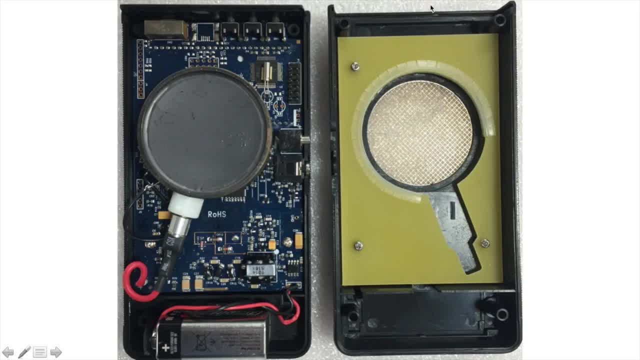 mica layer. If we open the detector, this is what you see. Again, this is looking from the back. so that's the mica window right there. that's the GM tube. this type of tube is called a pancake GM tube, but it kind of looks like a pancake. That's the. 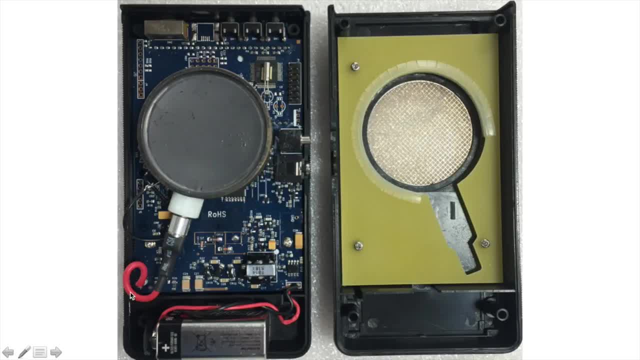 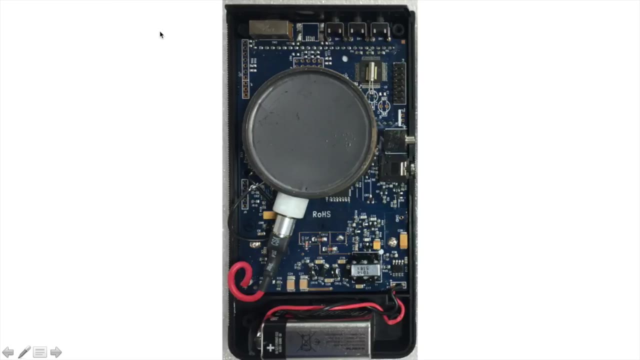 grid on the back of the box. Then you can see the anode connecting to the high voltage and the cathodes right here connecting to the ground through our resistor. You can see the switches on the top. This switch here is. let's look in more detail here. 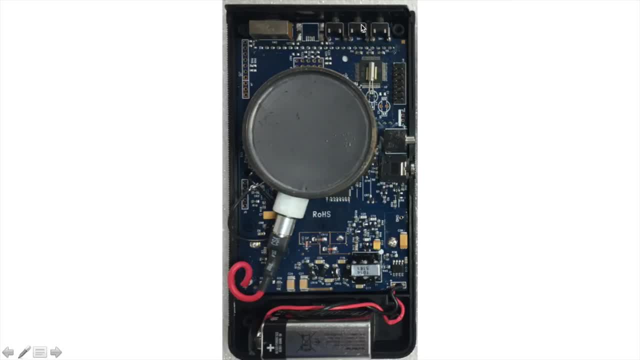 this switch is a timer. you have a setting plus or minus switch when you're programming the unit and there looks like a USB connector. there that's not mounted The processor, which is the main smarts of this device, with the crystal over there, These two audio jack. 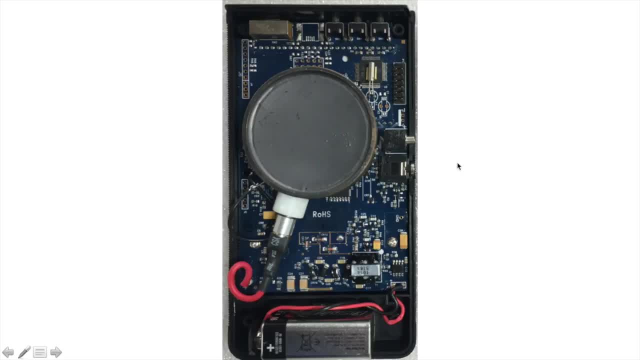 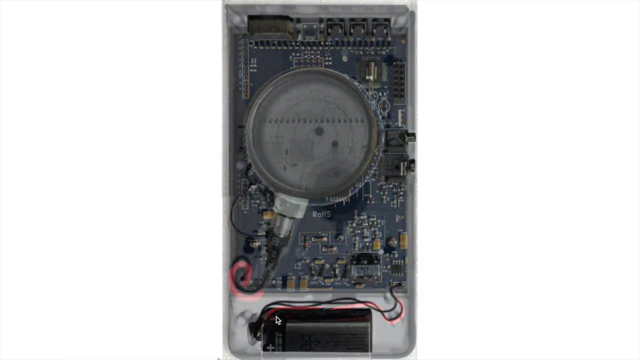 connectors here allow you to export the signal and also do calibration. The transformer and this unit here is the high voltage, using the ladder of capacitors and diodes here to create the high voltage that empowers the GM tube, and there is a 9 volt battery. Now, if we now take a look at the x-ray, that's how. 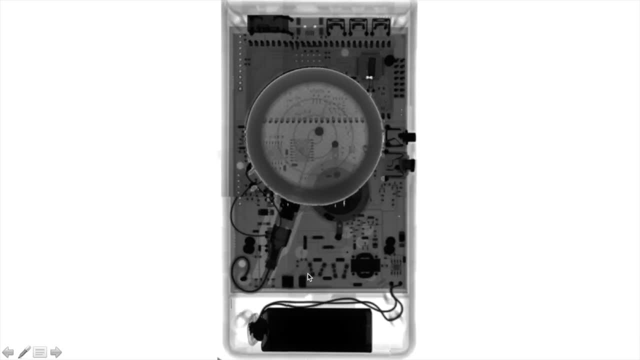 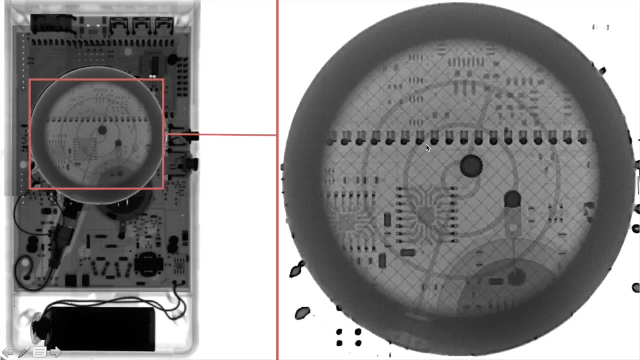 things look in the X-ray. So it's pretty cool. The high voltage unit. here let's look in more detail. You can see through the GM tube that grid that you see there looks like a bullseye. that's the grid for the anode. So that's where those 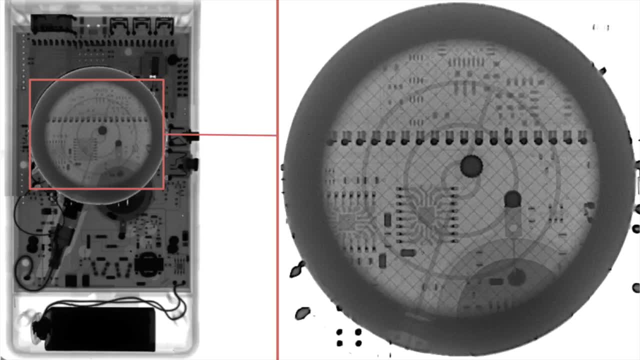 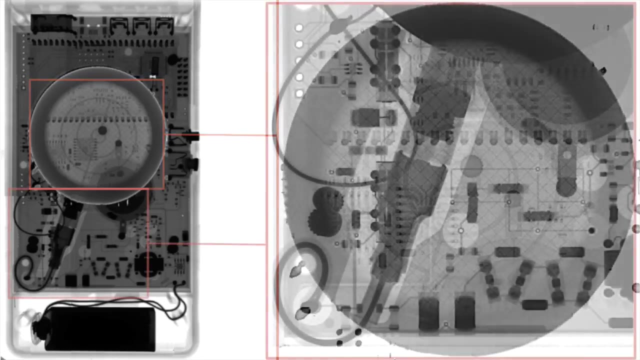 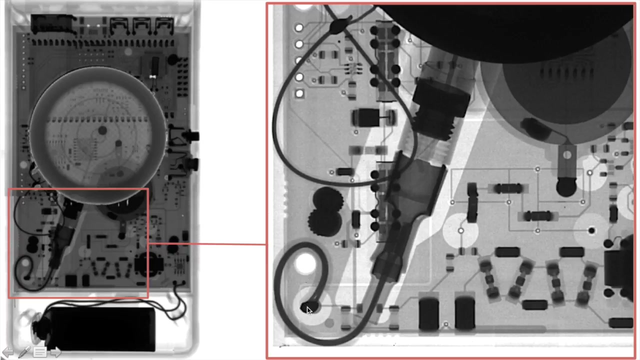 ionizing avalanche are colliding, So the anode is connected to create the signal. You can see how that then goes through inside the cathode to the outside of the GM tube and they go- that's the continuation of the anode- going through this wire. that 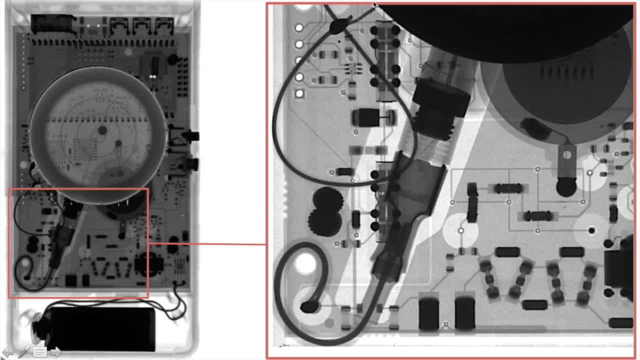 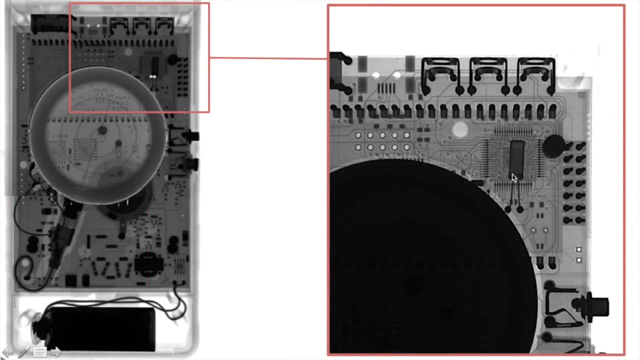 then connects to the high voltage circuit and the cathode goes on the other side. These are selection switches on the top that we saw before and this disk. here is the buzzer, basically the beep for the unit. And finally, here on the top we have- you can see in more detail- the processor, the crystal There's. 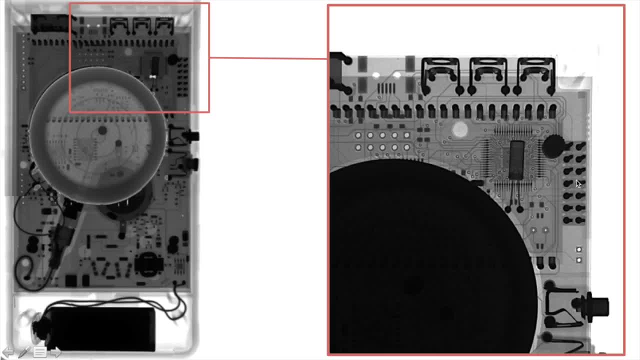 another connector here that doesn't have any access to the external world, so it's probably a programming, a JTAG type of connector to program this processor. These are the connections for the display over here and these are the selection switches. You can push buttons here on the top. Remember that the USB connector that's now.